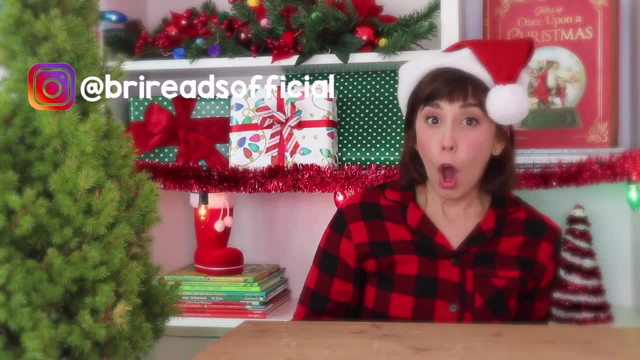 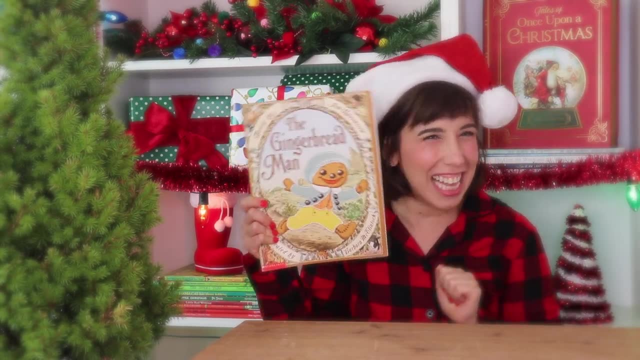 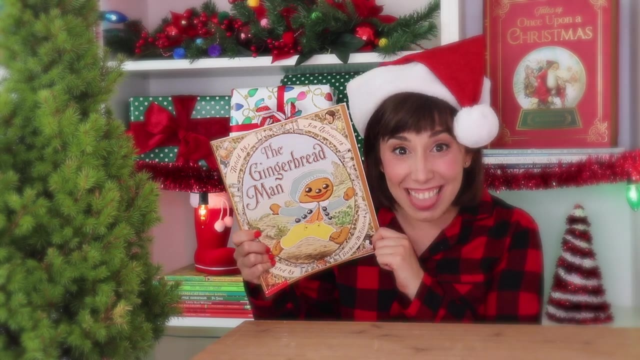 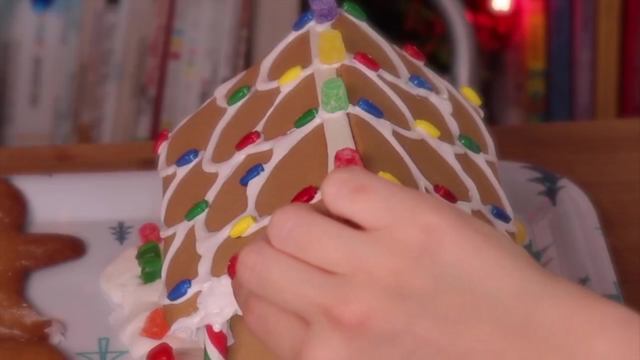 Do you follow me on Instagram? Over there, we read the story The Gingerbread Man- Run, run, run as fast as you can. You can't catch him. He's the gingerbread man. Today, let's make our own gingerbread cookies And later we can decorate a house for them with icing and sprinkles and candies. 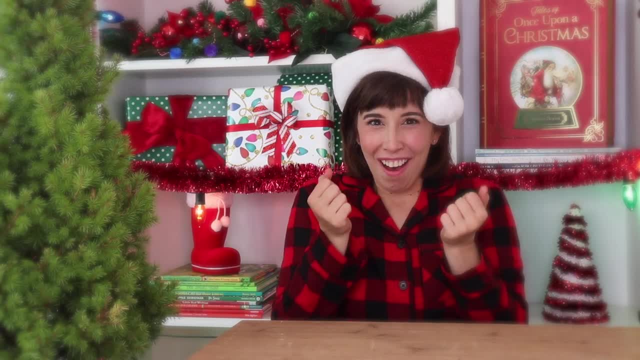 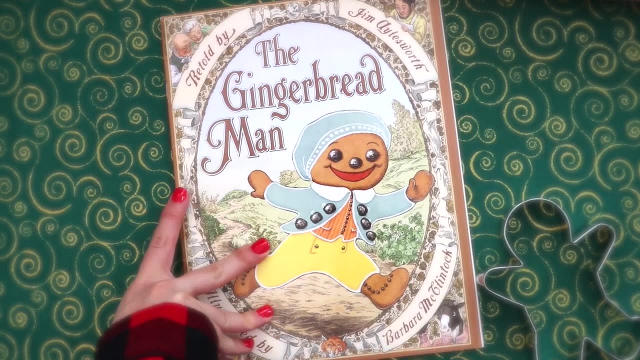 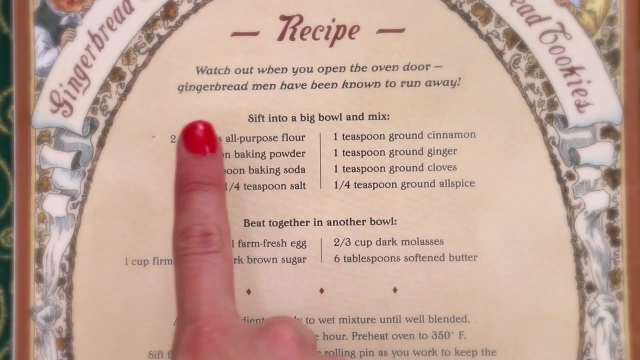 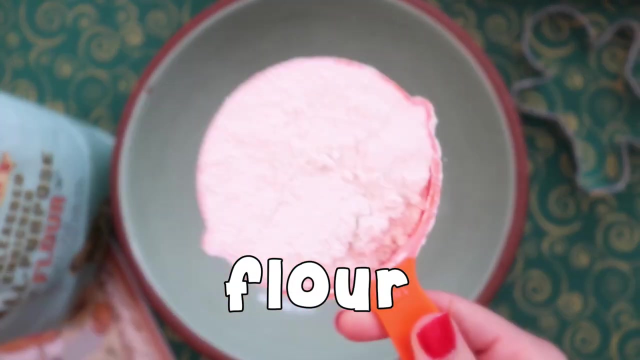 Friends, will you help me? Great, Let's get started. For this recipe, I'm following the one from The Gingerbread Man story. It's here on the back of the book. I read the ingredients one by one. First, the dry ingredients, like flour, baking powder, baking soda. 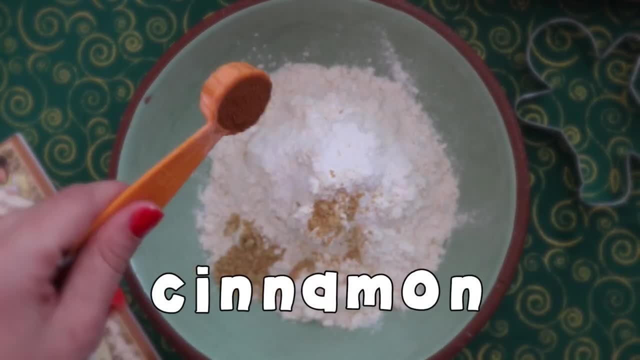 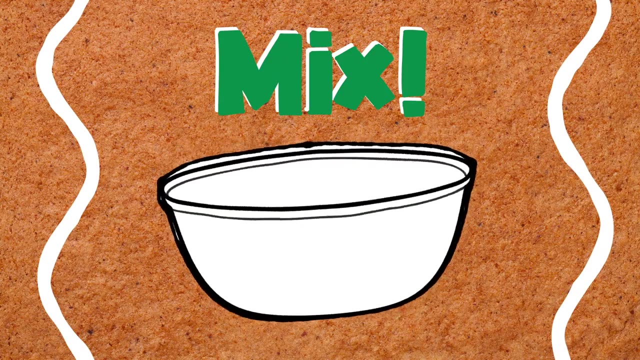 Then the spices for that delicious gingerbread taste: Ginger, cinnamon, cloves, allspice and a little bit of salt. Then the spices for that delicious gingerbread taste: Ginger, cinnamon, cloves, allspice and a little bit of salt. 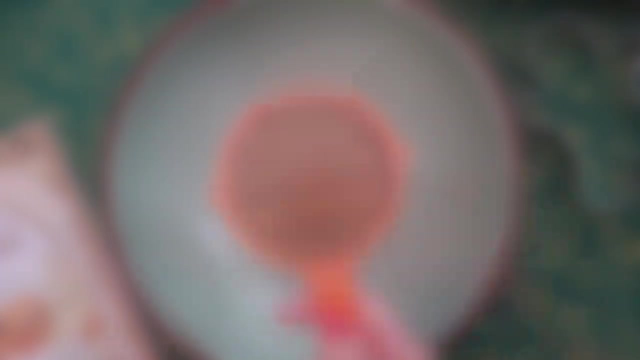 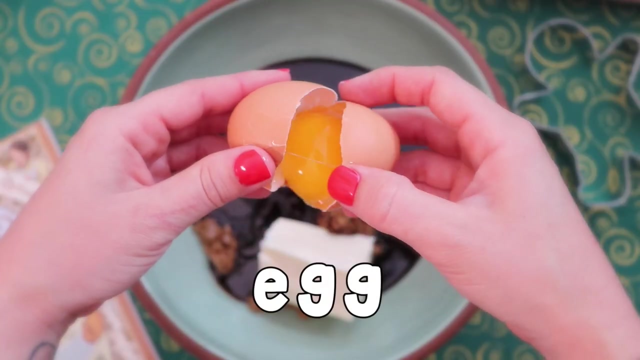 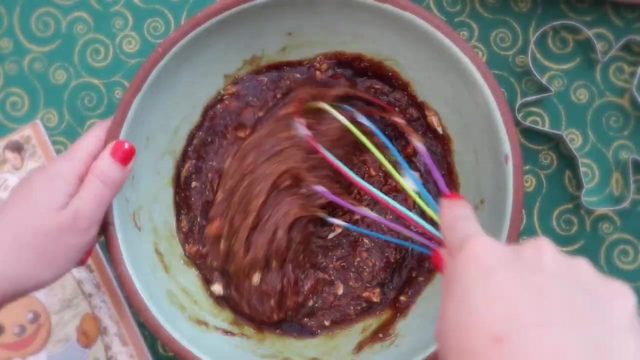 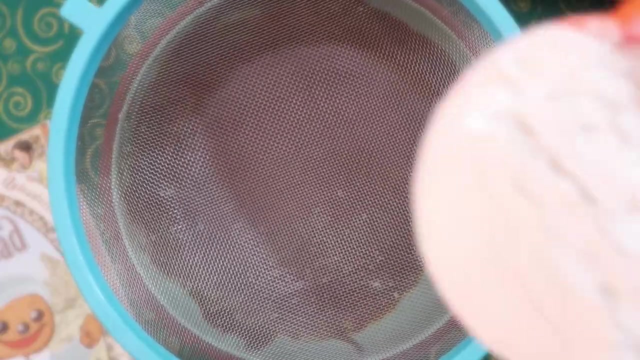 Mix it all up. I set those aside to prepare the wet ingredients: Brown sugar, molasses, butter and, last one, fresh egg Crack. Mix it all together. Now it's time to sift in the dry ingredients and mix one last time. 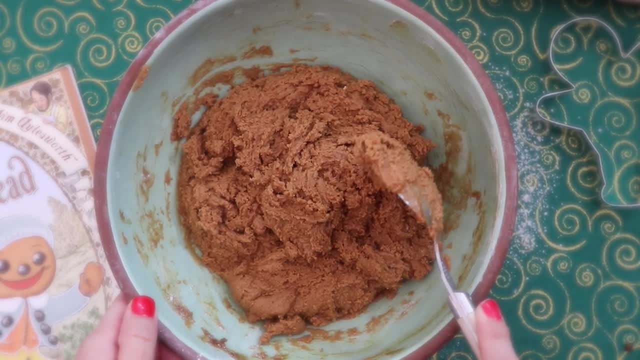 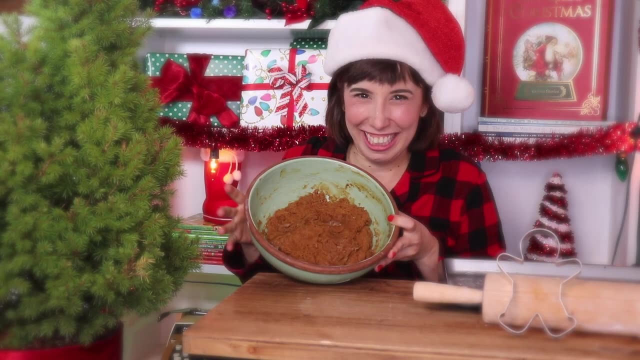 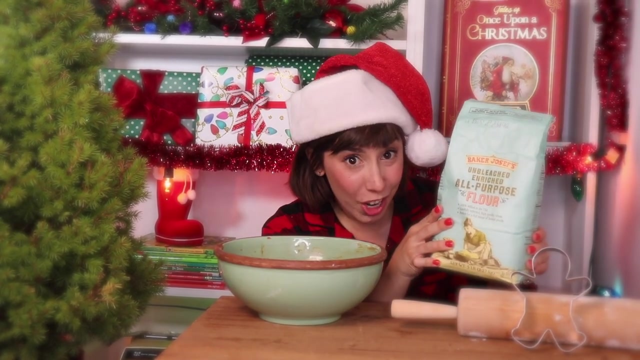 For the best results, I'll refrigerate the finished cookie dough for one hour. Now that the dough is finished, it's time to roll it out. Let's roll up our sleeves. This might get messy. We'll need plenty of flour. 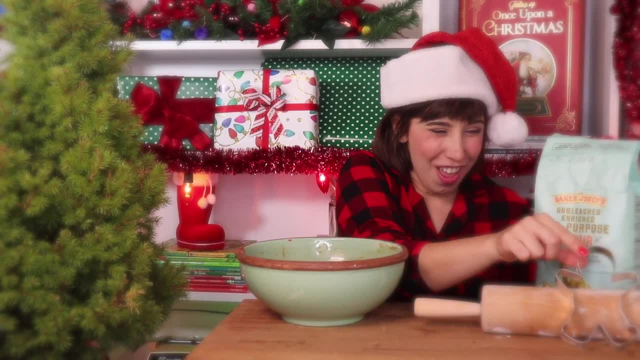 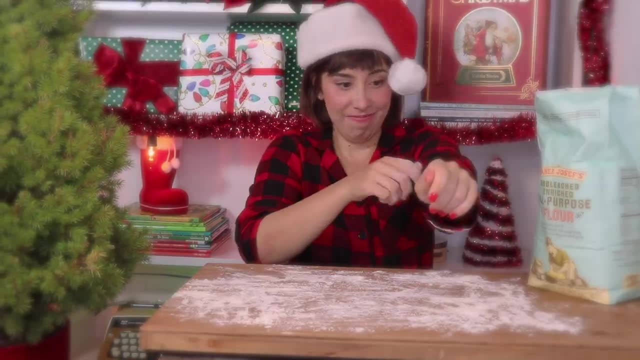 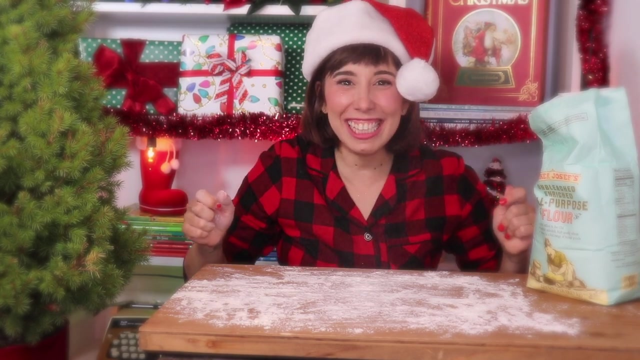 On my hands, on the rolling pin, on our little gingerbread cookie cutter and on the table. This dough is pretty sticky. Using flour helps it from sticking to everything. It looks like snow, Form your dough into a ball and plop. 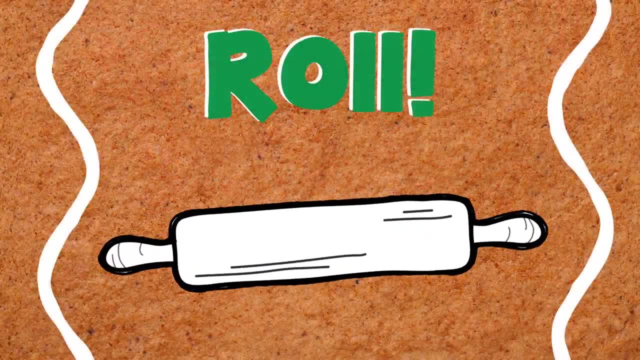 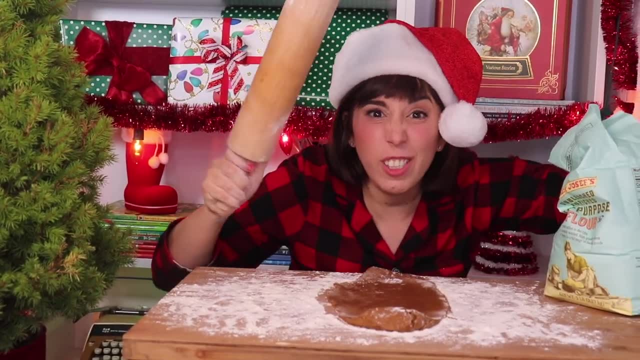 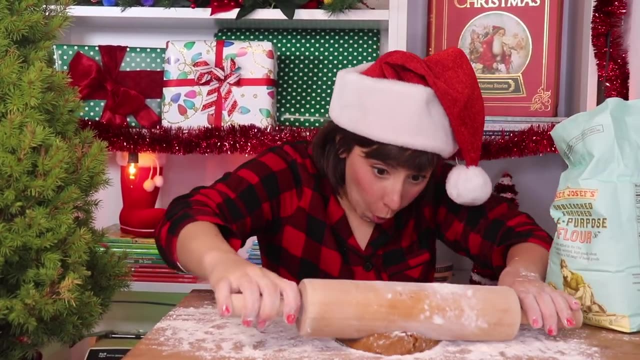 It's time to roll. First, you roll it, you roll it, you roll it, roll it, roll it If it starts sticking to your rolling pin. add flour, And then you roll, You roll it, you roll it, you roll it, roll it, roll it. 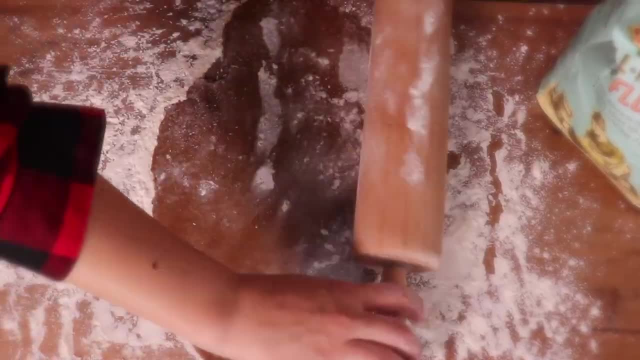 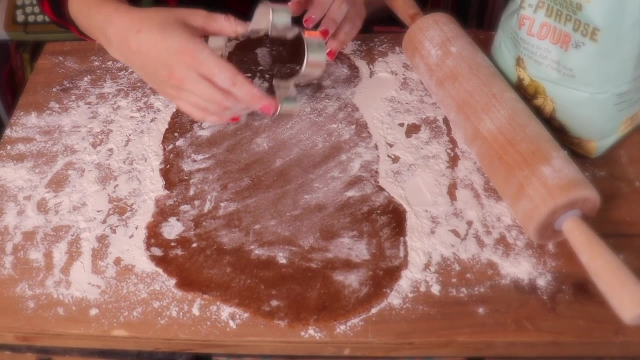 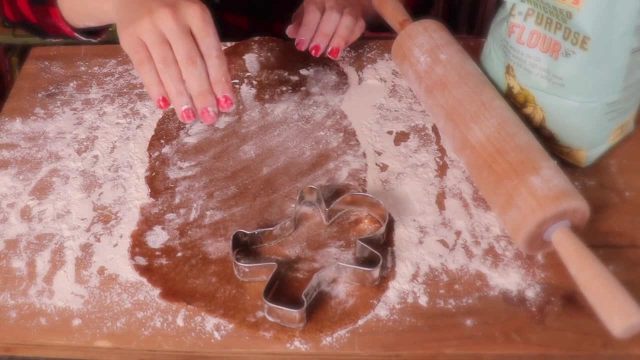 Until it's thin. I'm trying to push out the thicker parts, so it's all. even Next, you cut it, you cut it, you cut it with your cutter- Where does he fit This way? And then you push it, you push it, you push it and a wiggle. 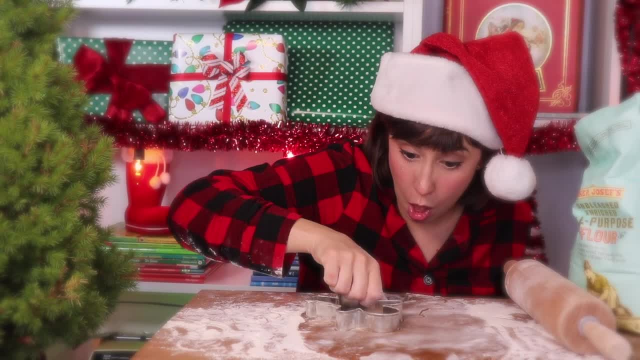 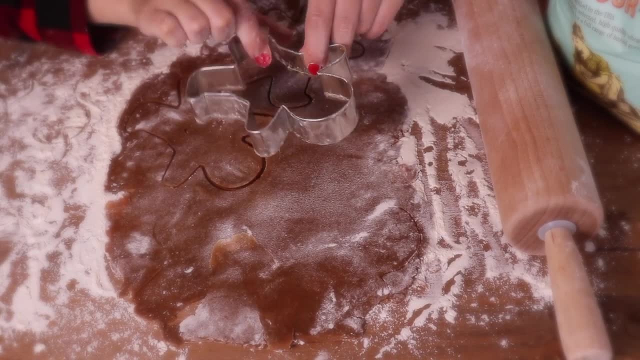 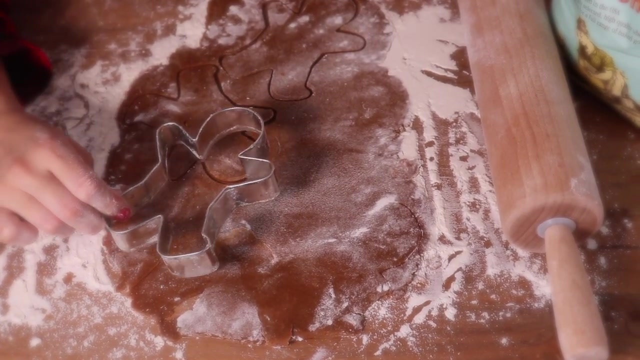 Again, It's just like a puzzle. Try to fit as many cookies on the same piece as you can. Let's see Where does it fit. Should it go here? No, How about here? Will that work? Yes, it's good. 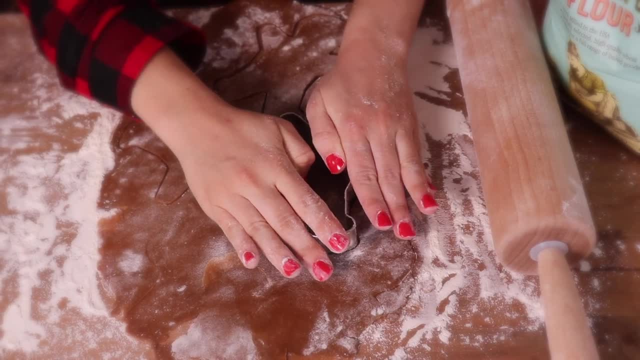 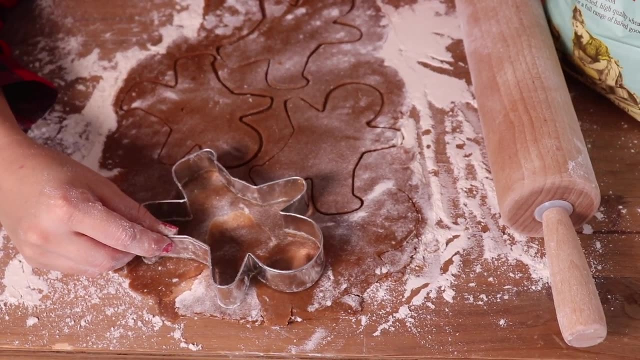 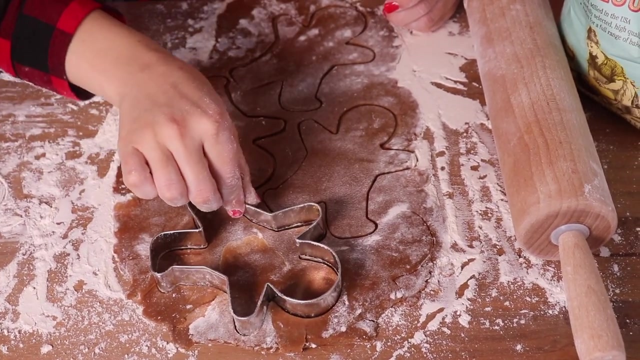 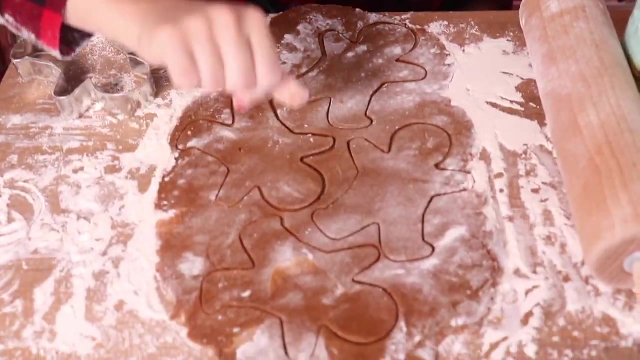 Let's push, Push down And lift. Can we fit one more? I think so. Let's push, Wiggle, wiggle, wiggle and lift. How many gingerbread did we make? Let's count One, two, three, four. 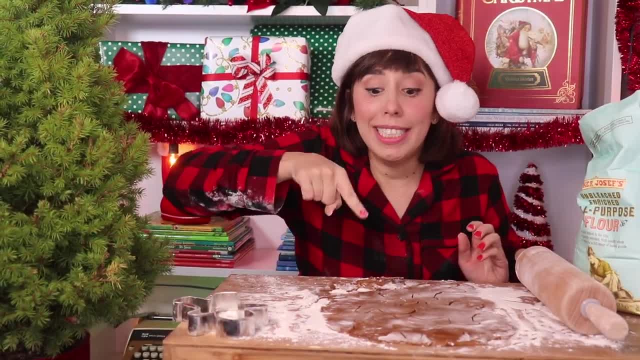 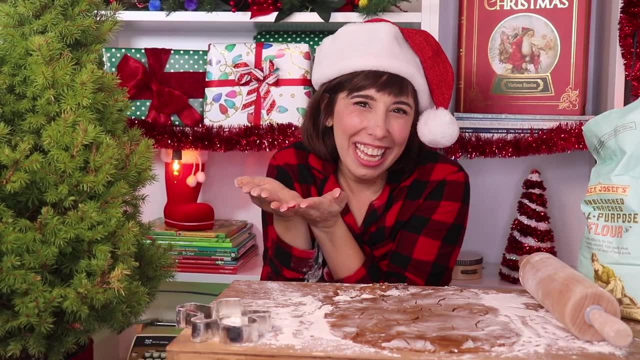 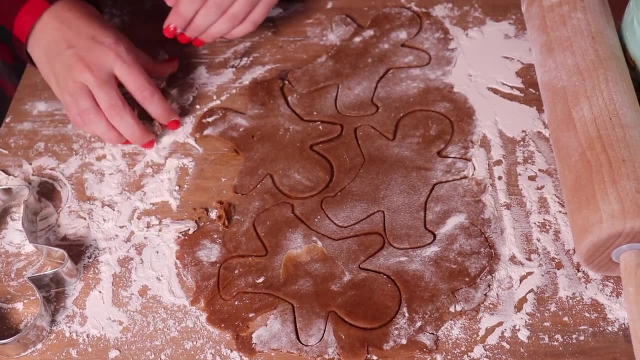 Four gingerbread cookies. Now we take away all the extra dough and load our gingerbread cookies onto the pan for baking. The best part is, you can use all this extra dough again. Just put it all together in a ball and roll it once more. 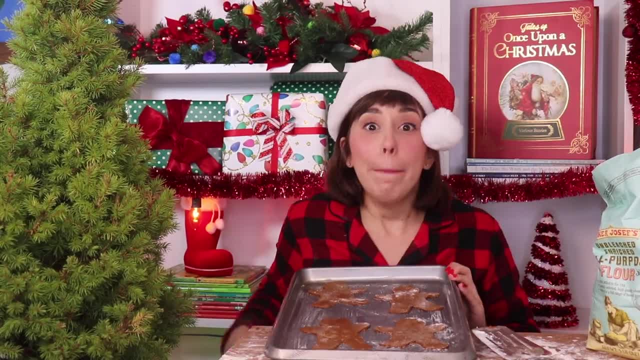 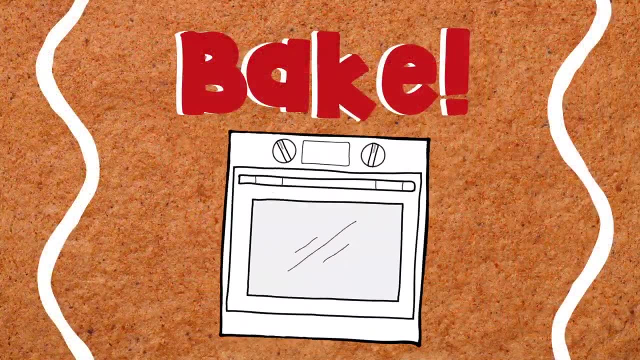 Now our friends are ready to be baked. Make sure to get a grownup's help to put them in the oven. It's time to bake Ta-da. They're all done, But not quite ready to eat. They need decorations. And how fun is this? 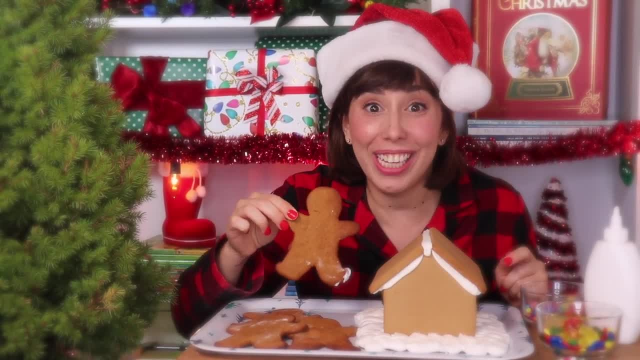